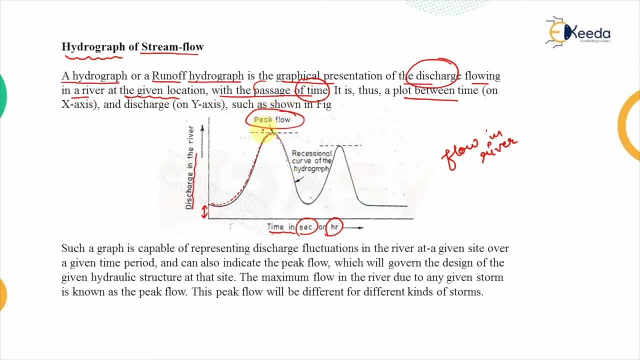 which is known as the peak flow, and the discharge corresponding to this peak flow is known as the peak discharge. then, as the rainfall recedes and the intensity reduces, then again it recedes down, and again, if the rainfall picks up or if the catchment is such that there is another area, 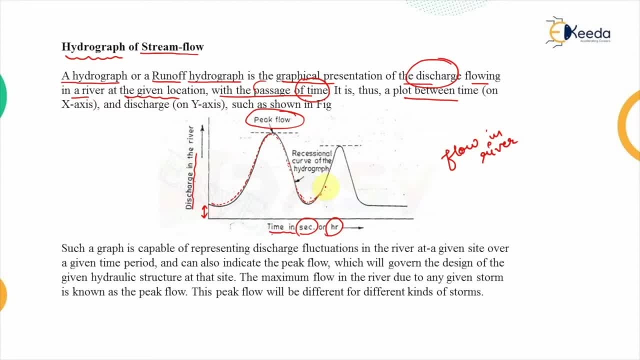 which is contributing towards the outlet point, but late. then again we will have the second peak, which will be staggered from the first one. now, what we are understanding from the hydrograph? that it is capable of representing the discharge fluctuations in the river at a given site for a given time period, and it also indicates the peak. 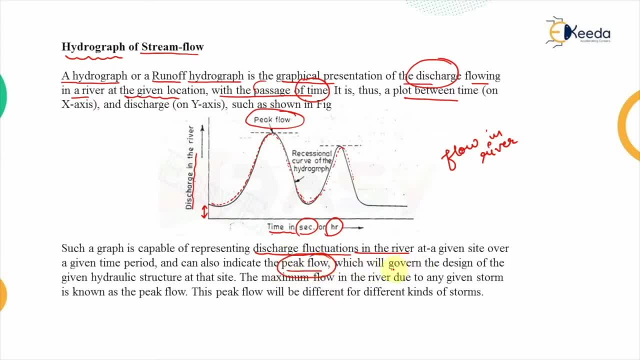 flow. now that peak flow is very important because it will govern the design of the given hydraulic structure at that site. so the maximum flow in the river due to that peak flow is very important. Now let's look at another example of a peak flow, which is known as the peak flow. 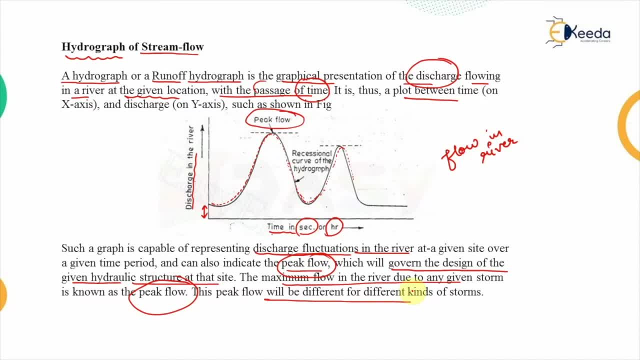 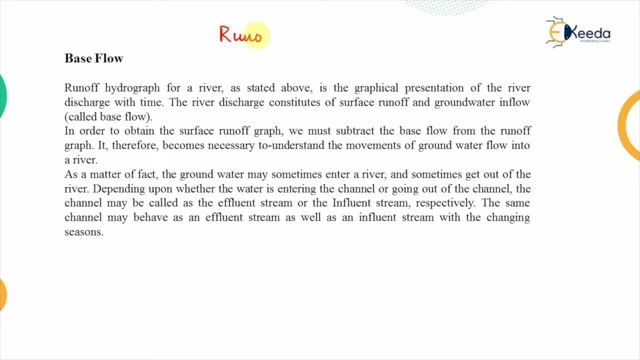 and it will be different for different kinds of the storm. then the base flow. so, as we have to date, that runoff, when we see it, is composed of the two components. first one is the direct runoff, second one is known as the base flow. now, the direct runoff is the one. 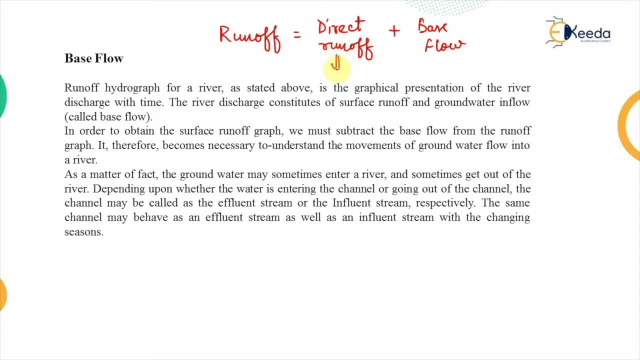 which we are looking in these streams directly, while this base flow is in the form of the ground water which is contributing towards the runoff, but very late Now, the runoff hydrograph, when we tell for the entire runoff, that is known as the flood hydrograph, because if the entire water is counted and if that is released simultaneously, 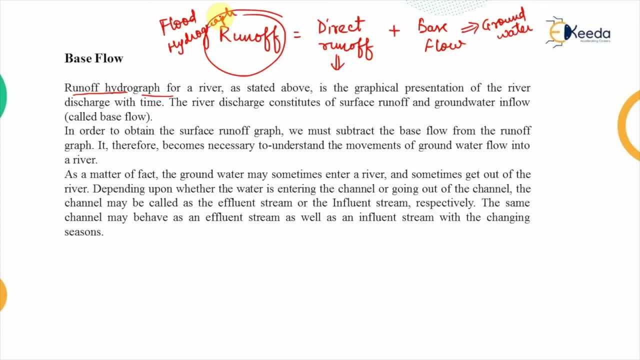 it will create the chances of the floodings. because of that reason, that particular hydrograph is known as the flood hydrograph, out of which a component is regarding the base flow, now the river discharge. it constitutes of the surface runoff, which we know as the direct runoff. 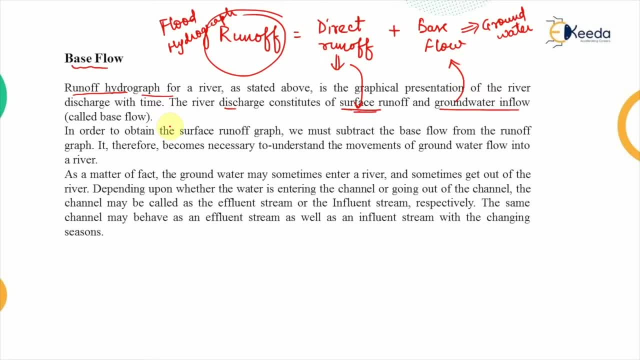 and the ground water in flow, which is known as the base flow. Now, if we want to obtain that, what is the actual contribution? because this base flow- let's say right now the rain is occurring, so that will be contributing directly towards this surface runoff or the direct runoff, but the base flow that was already present in the ground. 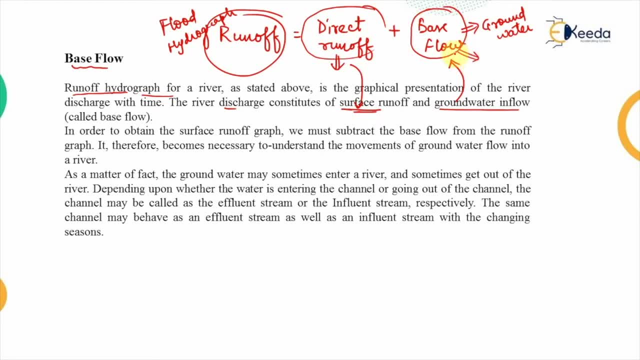 so it might be possible that this base flow that we are getting, it is representing the another rain fall which has occurred in the previous time. so to have a clear picture, to obtain the surface runoff graph, we must subtract the base flow from the runoff graph and therefore it becomes necessary. 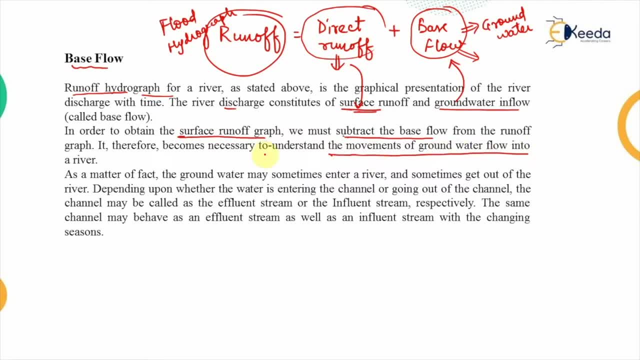 to understand the movements of the ground water flow into a river, that how the ground water discharges into the river. now, as a matter of fact, this ground water, it may sometimes be a surface runoff. it may sometimes enter a river or may sometimes get out of the river. that depends. 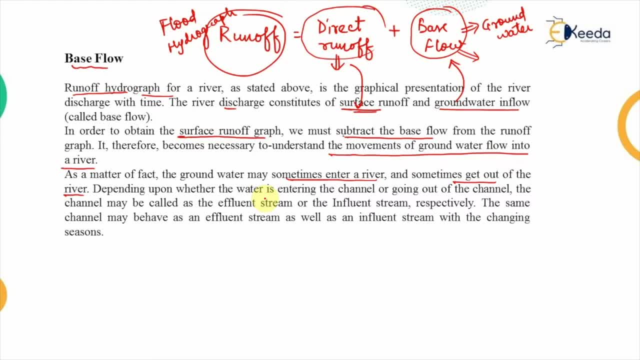 whether the level of the water in the river is above the water table or below the water table. now, if the water is entering the channel, then it is known as the affluent stream, or if it is getting out of the channel, then it is known as the influent stream. so the same channel it. 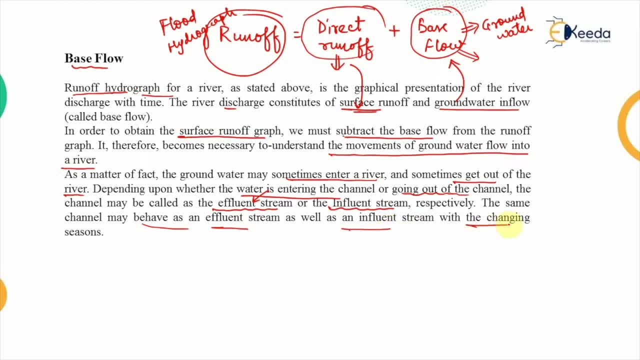 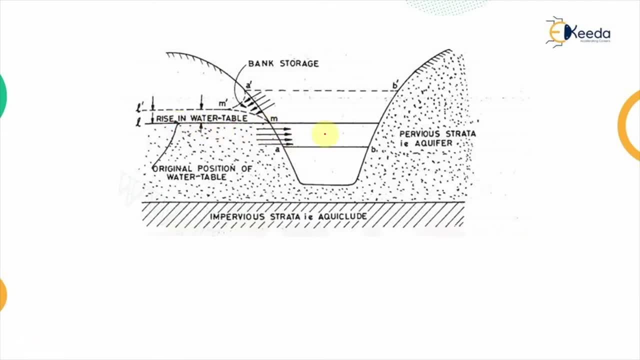 may behave as an effluent stream as well as an influent, with the changing seasons. for example, if you look at this image, this is the water table which was originally present. this is the water table shown with the red color. now, in the summer season, when the river is dry, this is the water level. so if the level 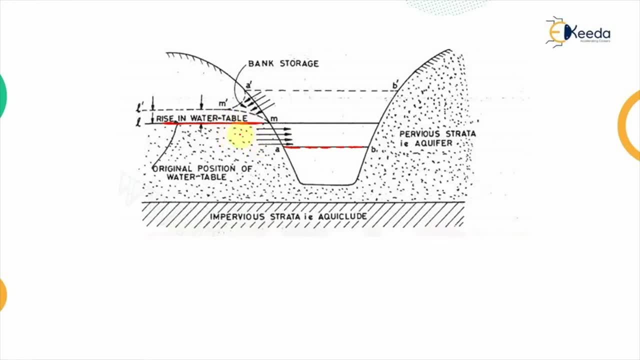 difference is present, then what will happen? the water will move from higher level to the lower level. so this will change the flow of water: from the lower level to the lower level, so this will be the direction of the water movement: from the groundwater to the river stream. 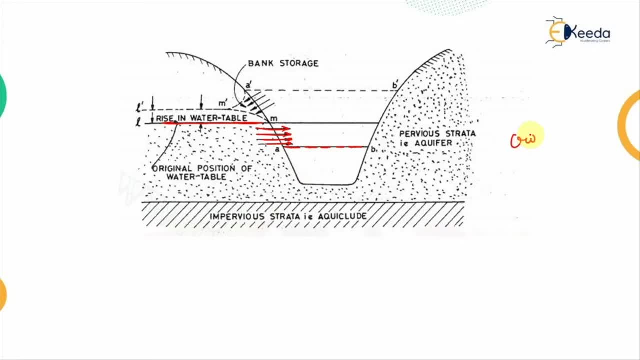 This is the cross-section of the river, so in this case, the water will be entering from the ground to the river. Now, if there is a rainy season, then the level of the water in the river that will increase up to this A dash, B dash level, which is higher than the level of the groundwater table. 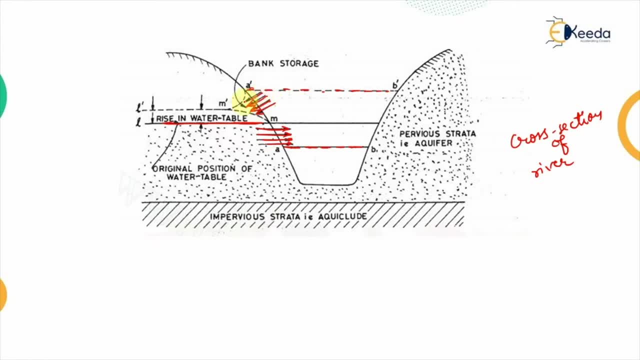 Because of the difference in the level of the water, the water will move from the river stream to the groundwater surface, Because of which there will be rise in the water table and, as you can see, when the water was entering into the channel, this was the affluent stream. 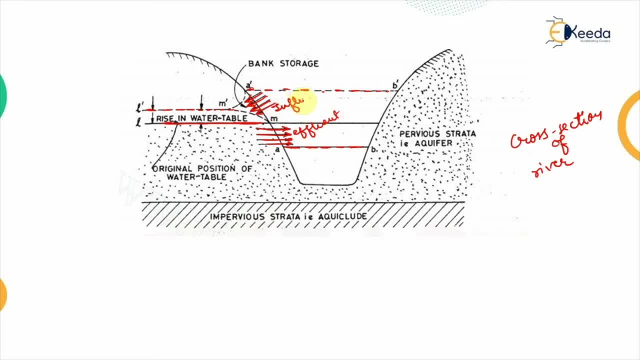 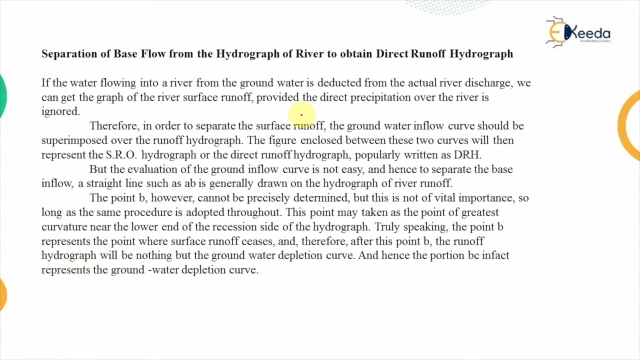 but when the water is exiting the channel, that is the influent stream, So the same stream may be the affluent as well as the influent one. So we have to deduct this ground flow because that might not be representing the true picture. Therefore, we need to separate the base flow from the flood. 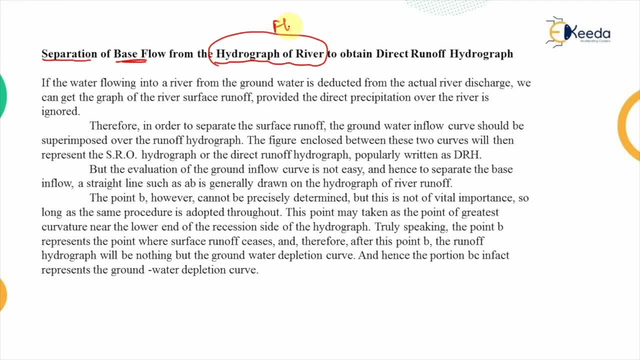 hydrograph, which is the hydrograph of the river. to operate the flow We need to obtain the direct runoff hydrograph or the surface hydrograph. So if the water flowing into the river from the ground, if that is deducted from the actual river discharge, we can get the graph for the surface runoff, provided. 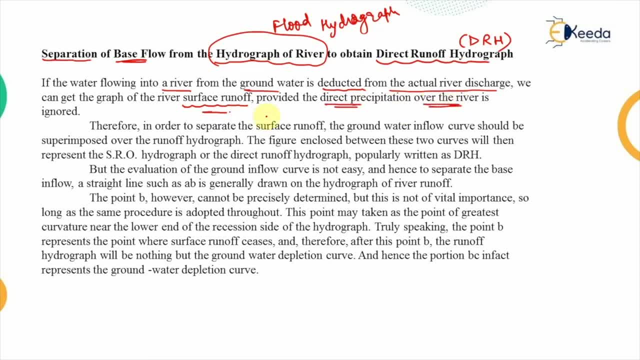 that the direct precipitation over the river that is ignored, and that is a very important assumption, Because what we are ignoring, that whatever rainfall is contributing directly towards the river, that is not counted. Therefore, in order to separate the surface runoff, the ground water flow curve that should. 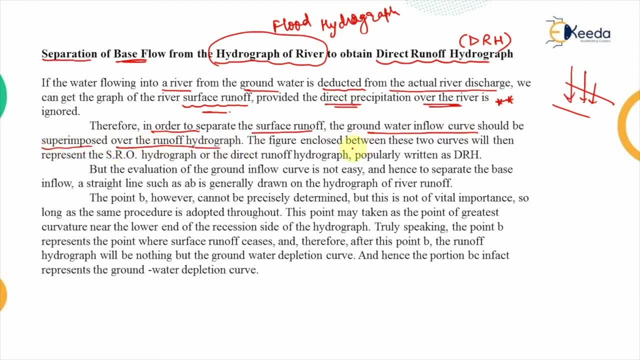 be superimposed over the runoff hydrograph, Now the figure enclosed between these two curves. it will be representing the surface runoff hydrograph, Which is also known as the direct runoff hydrograph, And in the coming lectures we will discuss this term only as DRH. that is, the direct runoff. 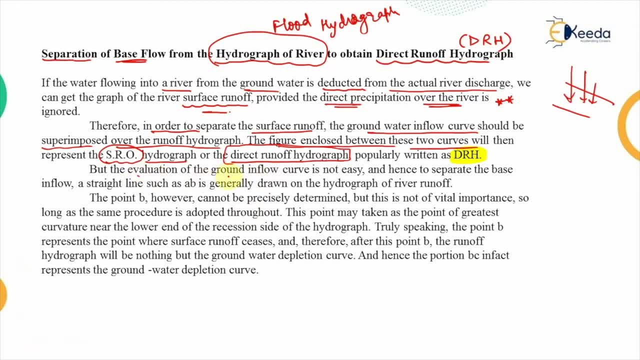 hydrograph. But this evaluation of the ground inflow curve, that is not easy because we were not having the data points for the ground inflow. Hence, to separate this base flow, a straight line, As shown in the next figure AB, is drawn on the hydrograph of the river. 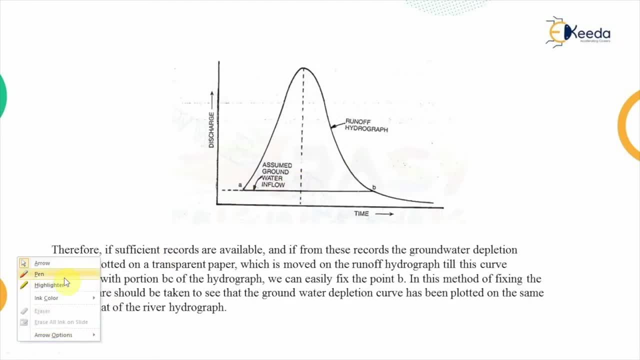 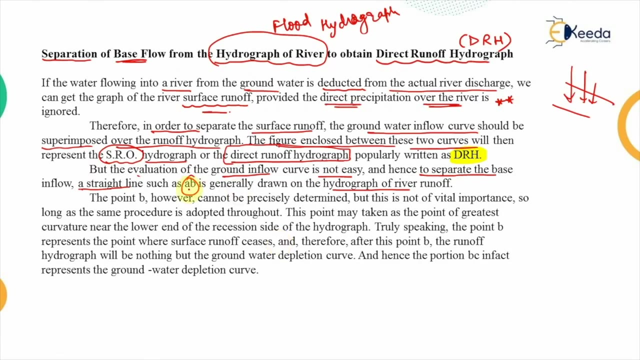 So, as you can see, this is a typical hydrograph which is obtained for the river flow. So this hypothetical line AB is drawn parallel to the time base. Now, this point B, it cannot be precisely determined, but this is not of vital importance, Because this point is taken as the point of greatest curvature, near the lower end of 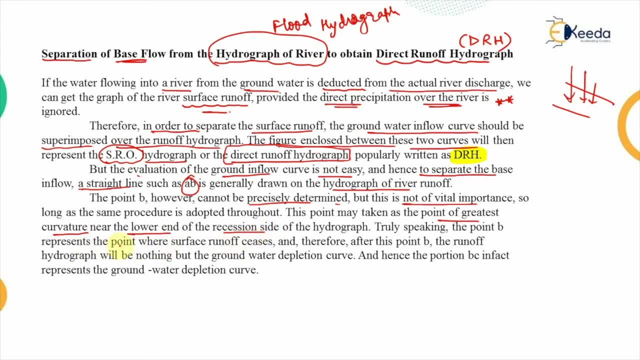 the recession site Because it is representing that location where the surface runoff, it ceases, where it stops, And after this point B, only runoff will be because of the ground water And it is representing the ground water depletion after that. Therefore, this portion BC is representing the ground water depletion curve. 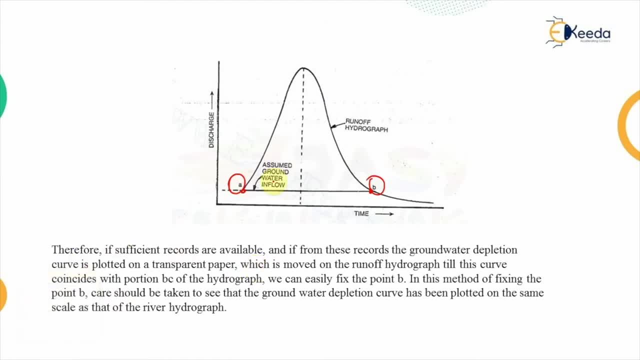 So from the entire river runoff curve. if we subtract this base flow, the remaining one that we will be getting, that is known as the direct runoff hydrograph. That means the water from the precipitation which is contributing directly to the water flow towards the surface runoff. 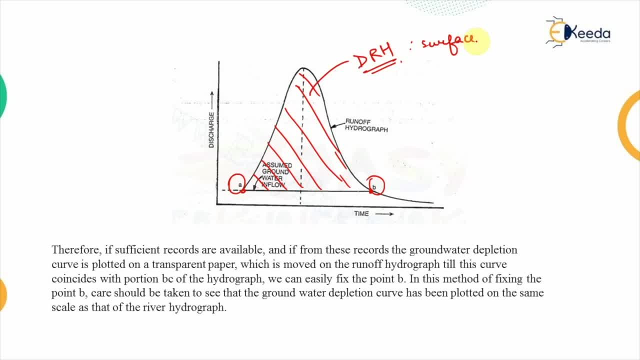 And this surface runoff that is contributed from the portion of the precipitation which is known as the excess rainfall. That was after deducting the discharge basin, the initial basin recharge and the soil moisture deficiency. The remaining one was the excess rainfall And that is equivalent to direct runoff hydrograph. 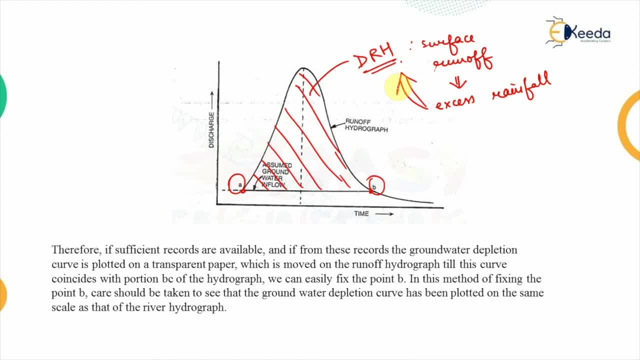 In response of it. Therefore, if the sufficient records are available and from those records the ground water depletion curve is plotted on a transparent paper, that it will be moved on this hydrograph. till this BC portion. This is B and C portion is coinciding.